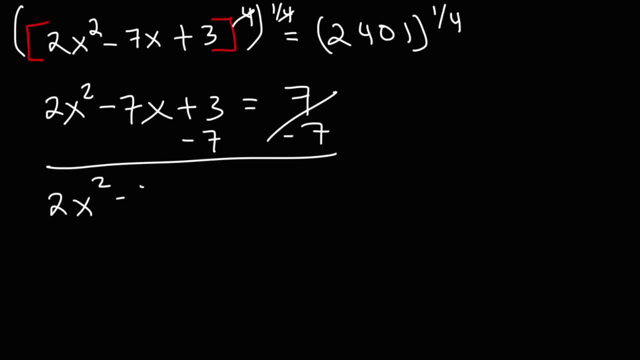 So we're going to have, So we're going to have, So we're going to have: 2x squared minus 7x minus 4 is equal to 0.. So what we now have is a quadratic equation. We have a trinomial where the leading coefficient is not 1.. 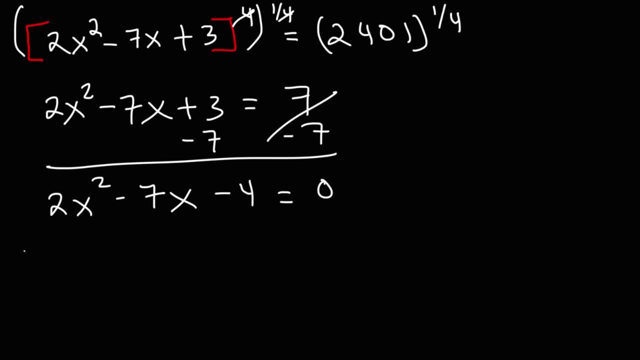 What do you think we need to do here In order to solve this equation? we could use the quadratic formula or we could try to factor it. I think we should definitely try to factor this equation. So here's what you need to do. 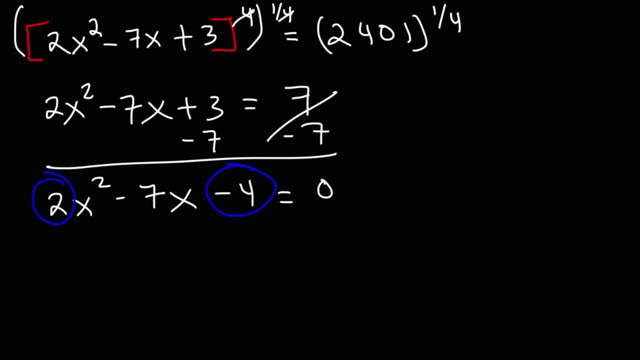 Multiply the leading coefficient 2, by the constant term negative 4.. 2 times negative 4 is negative 8.. And then find two numbers that multiply to negative 8, but add to negative 7. So we know that 2 and 4 can multiply to 8.. 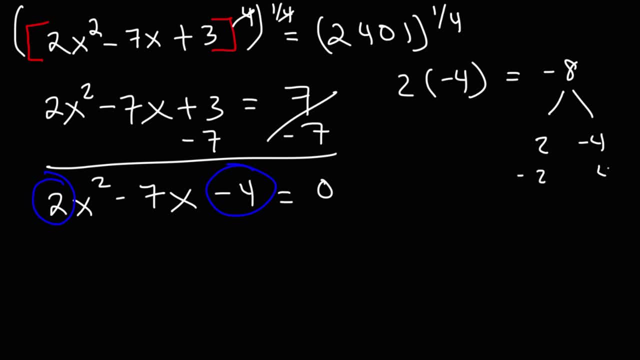 We can use negative 4, or we can use negative 2.. But none of these will add up to negative 7.. We could try 1 and 8.. We can try 2 and 8.. We can try negative 1, positive 8, or positive 1, negative 8.. 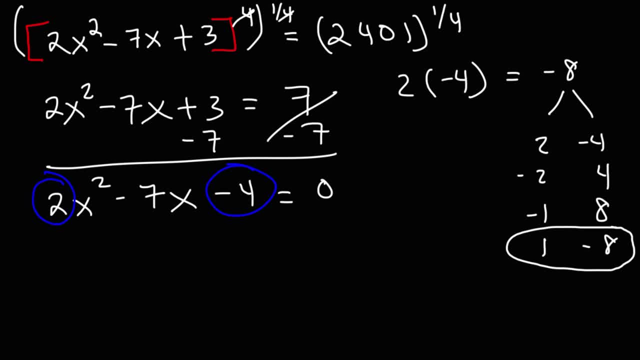 Now positive 1 and negative 8 adds up to negative 7. So we're going to use that. Let's replace negative 7x with negative 8x and positive 1x. So that's what we have right now. 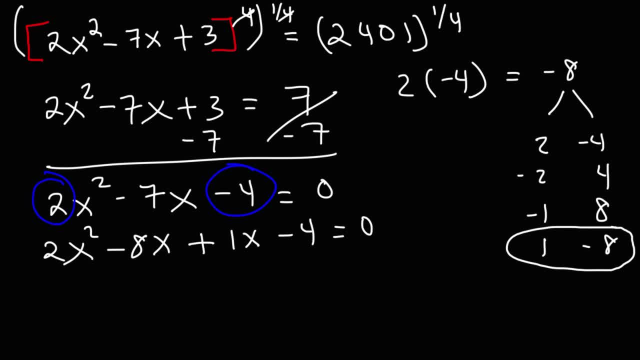 Now what we need to do is we need to use a technique called factoring by grouping. We need to take out the GCF, the greatest common factor out of the first two terms, And that's going to be 2x. 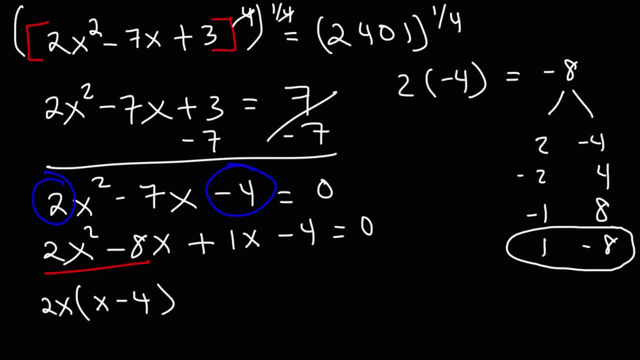 And it's going to leave behind x minus 4.. Now for the last two terms. the only thing we can factor out is 1,, which will also leave out x minus 4.. Now the next thing is to factor out another GCF, which is x minus 4, in this case. 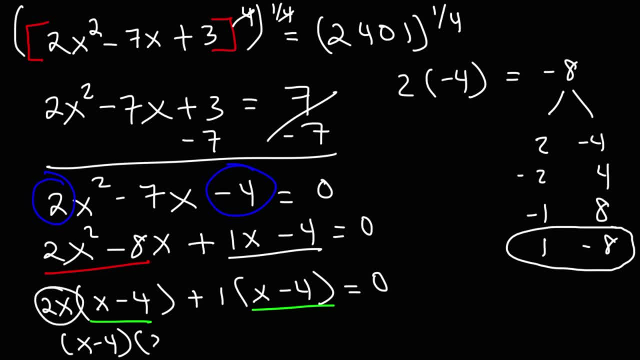 In front of the first term we have 2x, In front of the second one we have a plus 1.. So it's going to be x minus 4 times 2x plus 1. And that will equal 0.. 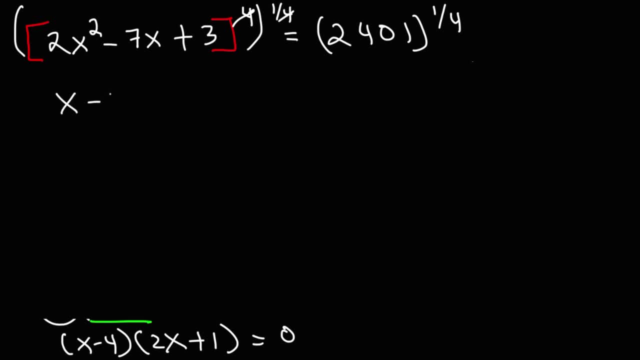 So now let's solve the equation. What we're going to do is we're going to use the zero product property and set each factor equal to 0.. So we're going to set x minus 4 equal to 0 and 2x plus 1 equal to 0.. 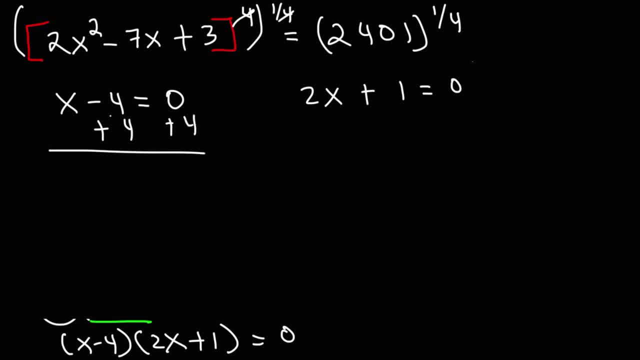 So add in 4 on both sides, And the first equation will give us our first answer, And that is that x is equal to 4.. And then for the second one, we're going to subtract 1 from both sides, So we'll get 2x is equal to negative 1.. 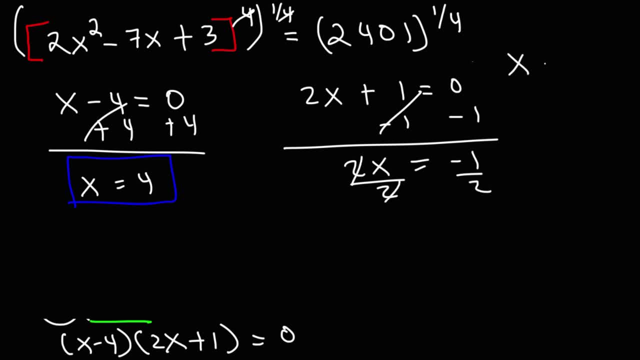 And then we're going to divide both sides by 2.. So we get the second answer. x is equal to negative 1 half. Now what we need to do is check the solutions to see if both answers are correct or if one or none of them is correct. 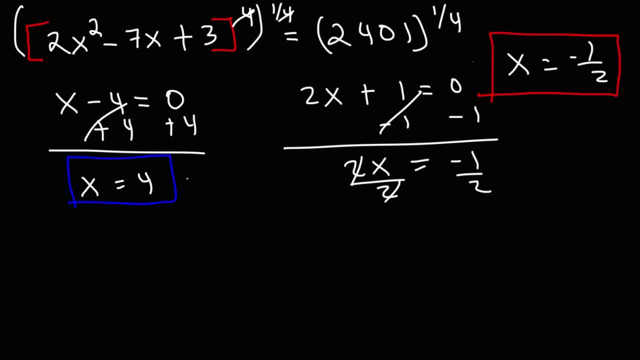 So let's begin by plugging in x equals 4 to the original equation. So replacing x with 4, we're going to have this 2 times 4 squared minus 7 times 4 plus 3.. All of that is going to be raised to the fourth power. 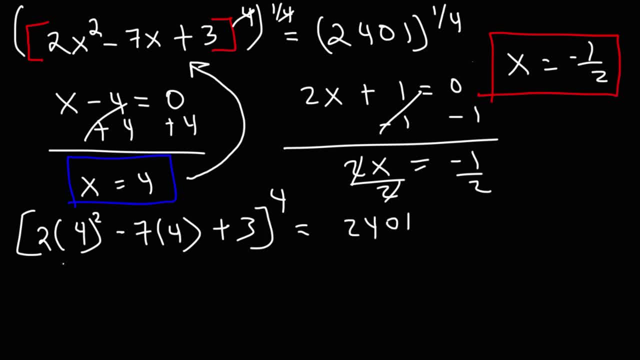 And we're going to see if it's equal to 24 or 1.. So 4 squared is 16 times 2,, that's 32.. 7 times 4 is 28.. And then we have 32 minus 28,, which is 4.. 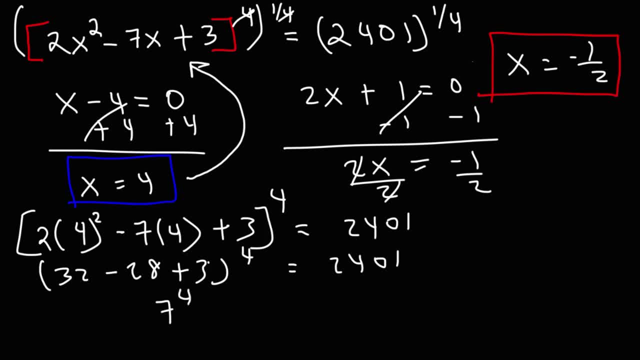 4 plus 3 is 7.. And so we get: 7 to the fourth is equal to 24 or 1.. And we know that is true. 7 to the fourth is 24 or 1.. So the first answer is correct. 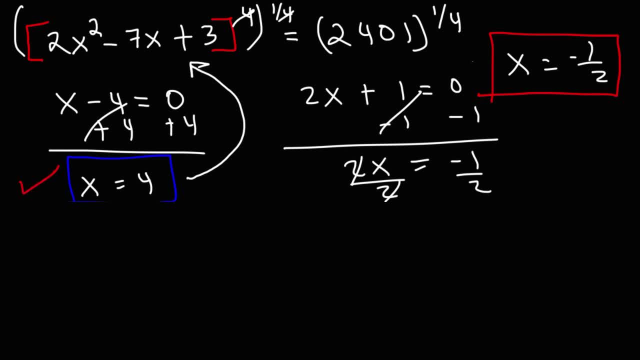 So let's put a check mark for that. Now let's see if our second solution is correct as well. So we're going to plug in negative 1 half. So this is going to require some work. So negative 1 half squared. 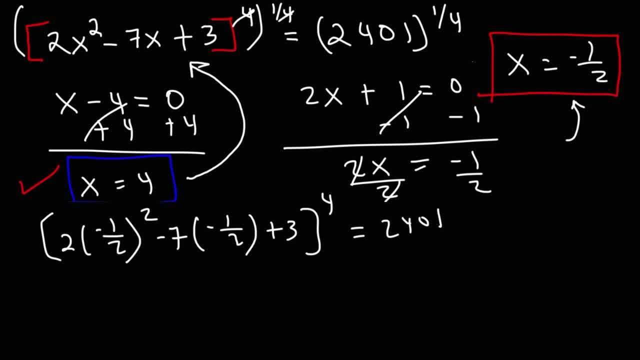 Negative. 1 squared is going to be positive 1. 2 squared is 4.. So we're going to have 2 times 1 over 4. And then this is going to be plus 7 over 2. And then plus 3..